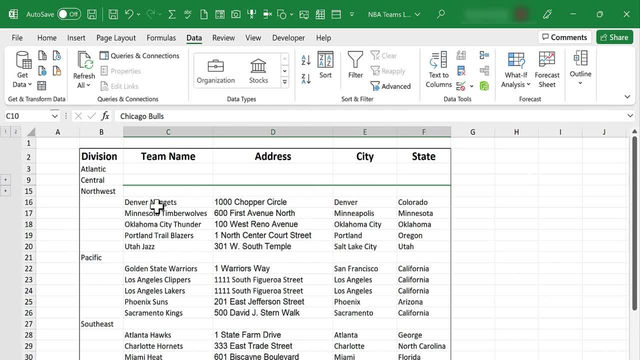 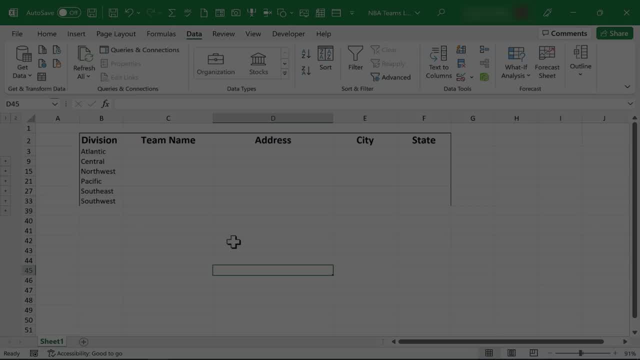 dialog box that pops open. I'm going to choose rows, Click OK. Now I can collapse the central division, So give me a minute to finish doing this for each of the divisions and then I'll resume the video. Okay, great, I've finished grouping all of the NBA teams based on their 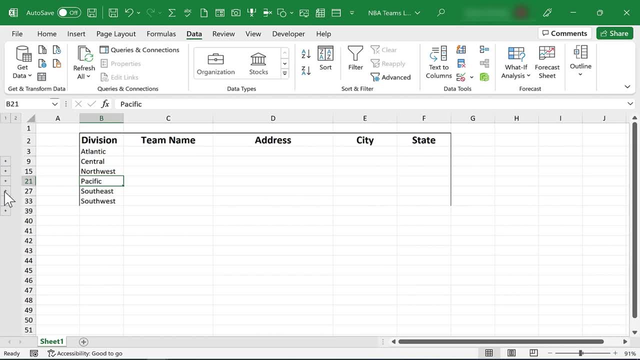 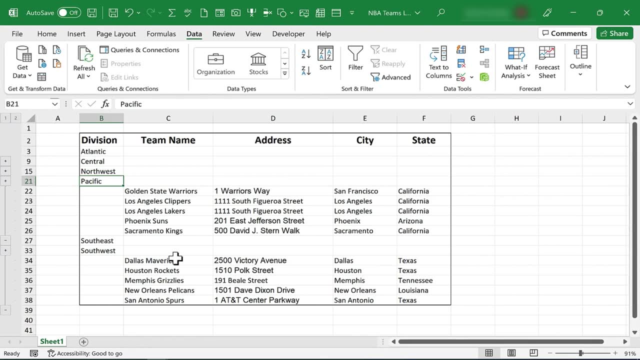 divisions. So now let's say I'm interested just in the Pacific division, I click the plus sign here and all of those teams are revealed. If I'm interested in the Southwest division, I click here and all of those teams are revealed. And again I can collapse those just by clicking. 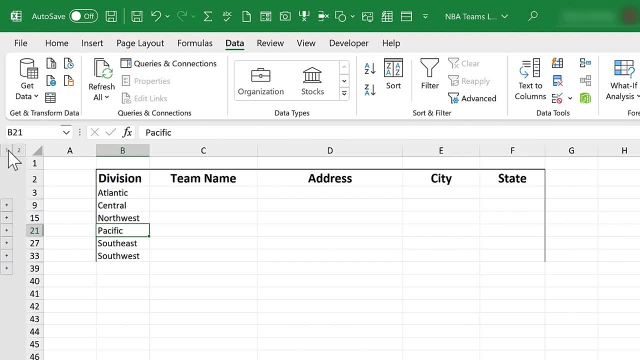 the plus sign. Now, here in the upper left corner, we also have some buttons that we can click. There's a number one. If you click the number one, it takes you to this top level where it just shows the list of divisions. If you click on two, it expands everything. So I can quickly collapse. 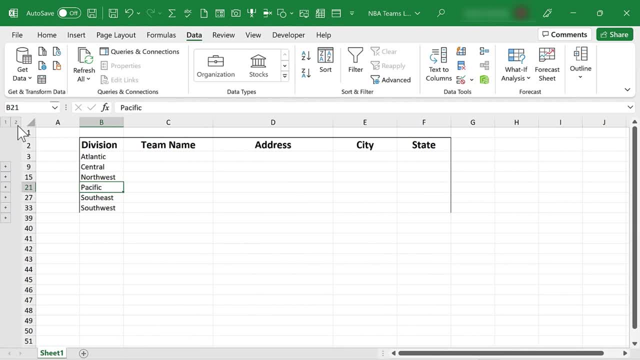 everything and expand everything by using these two buttons in the upper left, Or I can use these individual buttons here to collapse each division one by one that I would like to collapse, And that way I can see the specific information I'm looking for. So I'm going to go ahead and click collapse. 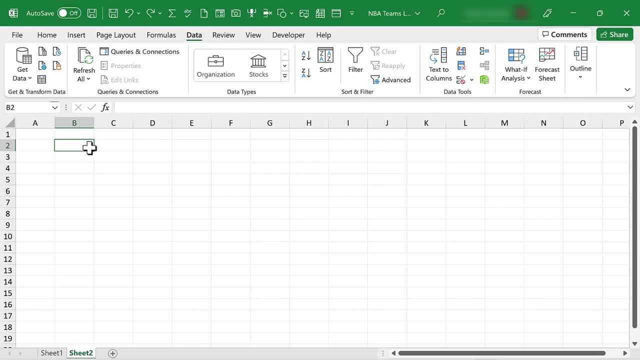 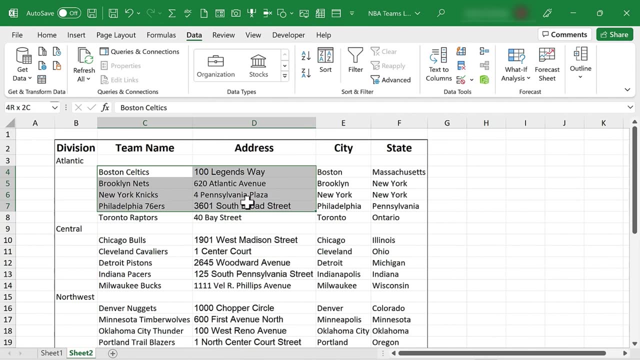 Now, in addition to grouping based on rows, we can also group based on columns. So I've copy pasted the same data onto a new tab. If I now select all of the teams in the Atlantic division, I can hold alt, shift, right arrow, But this time I'm going to group based on columns. I click ok. 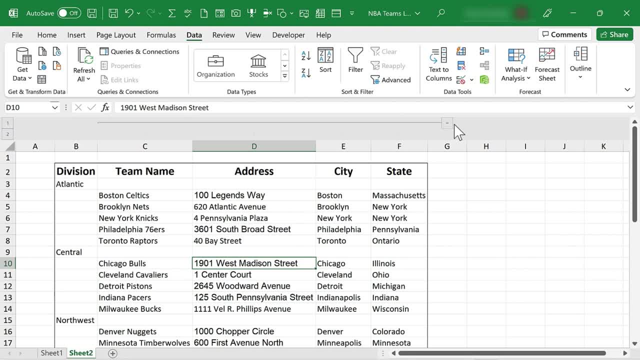 And now my data is collapsible in a different way. Up here at the top there's a minus button And you can see. in this case it doesn't make a lot of sense to collapse columns, But I just wanted you to see that that is possible and to get a glimpse of how that works. 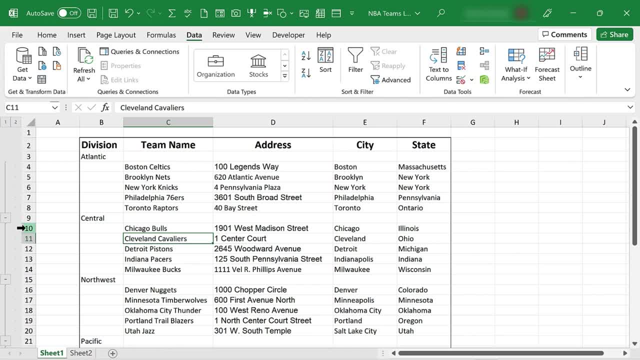 Jumping back to sheet one, what would I do if I wanted to remove these groups that I've created? All I would need to do is click and drag to select the range that I want to stop being a group And then go to the data tab- data ribbon- Here on the outline button. 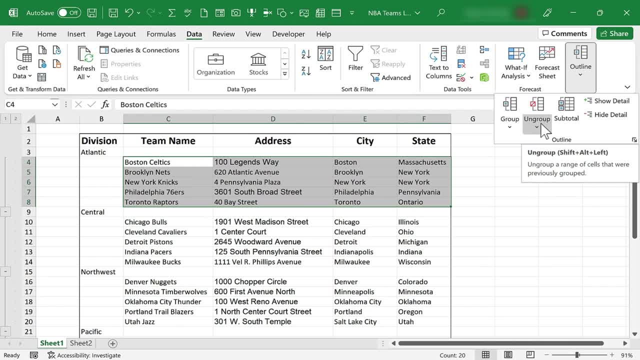 I'm going to click And you can see, in addition to group, there's also an option to ungroup. So I'll just click there. Do I want to ungroup the rows or the columns? And I click ok. And now you can see my line here at the left is gone. 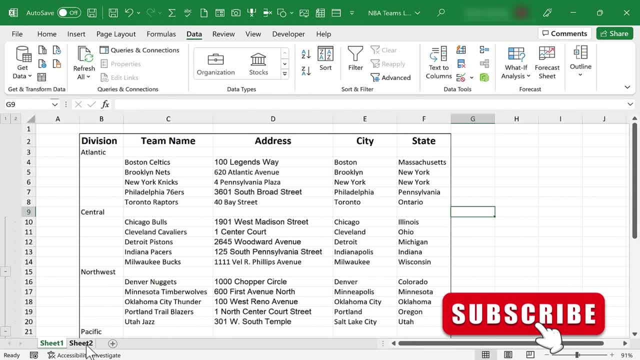 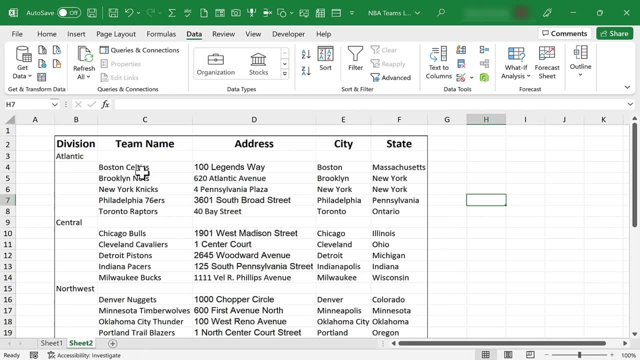 because this range is no longer grouped. One last thing that I want to point out here: on my second sheet I'm going to ungroup the columns that I had grouped And I want you to see that there is an option that we have on the data tab here on the outline. 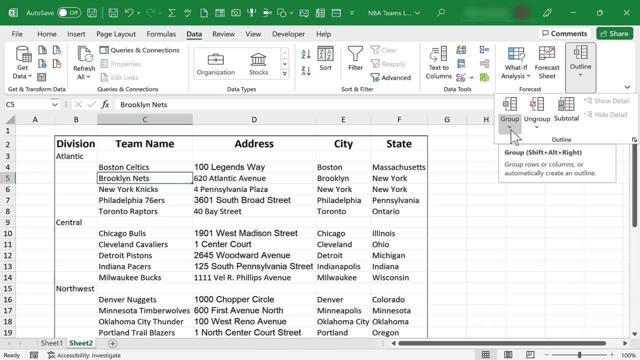 button. If you click there, there is an option for grouping. If you click here on the arrow- not on the button itself, but the arrow- there is an option to try to do an auto outline. Now, this sometimes works and it sometimes doesn't. I don't think it's going to work in this. 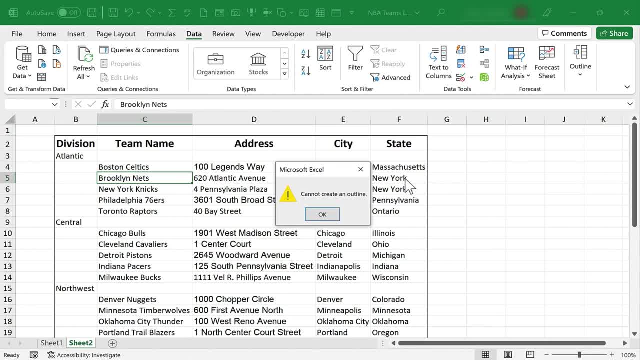 case, But you can try it. So I'm going to click here: auto outline. It says: cannot create an outline. So that's something that you can try if you would like. Doesn't always work. When it does work, what happens is Excel will automatically apply groups to the spreadsheet based on its 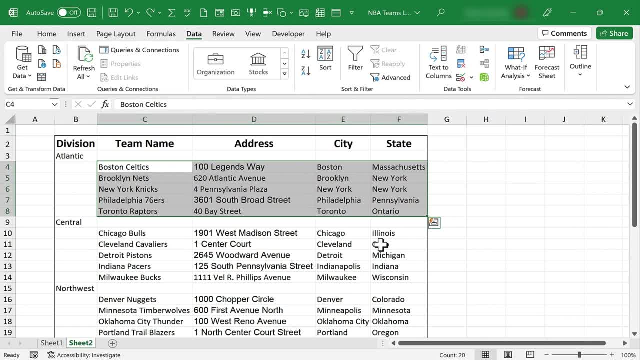 own logic, its own reasoning. Sometimes it works well, sometimes it doesn't. Now one last tip that I have for you when it comes to grouping rows or columns in Excel. I've taught you how to do this. You can use the shortcut key for grouping rows or columns. You click and drag. 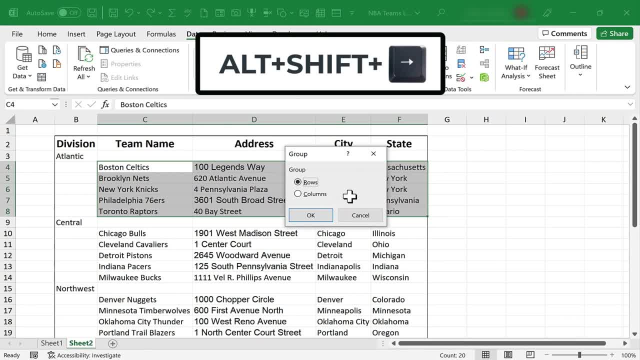 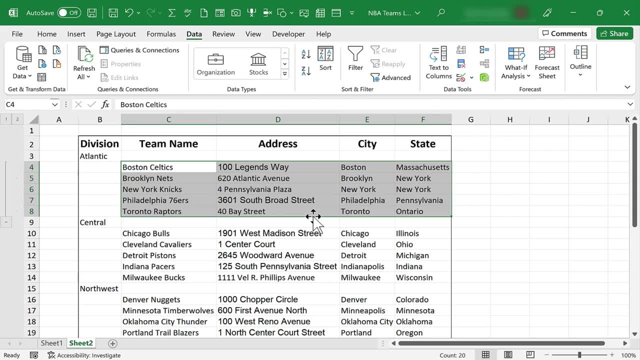 to select the range that you would like to group: Hold alt, hold shift, tap the right arrow and then choose rows or columns. Okay, fine, That's working great, But there's also a keyboard shortcut for removing the group. You can probably guess what it is: It's alt, shift, left arrow And. 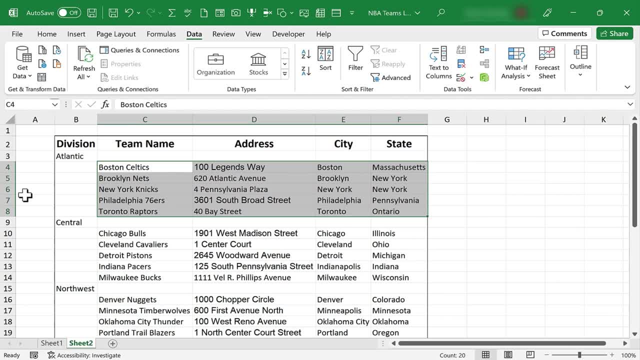 then you select rows or columns, click okay and that group is removed. So I hope you can see the potential that this technique has in your Excel spreadsheets. You can use it to organize your data, to make it easier for people to read and to find the 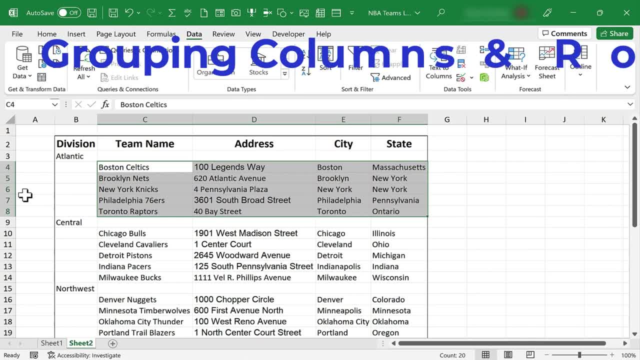 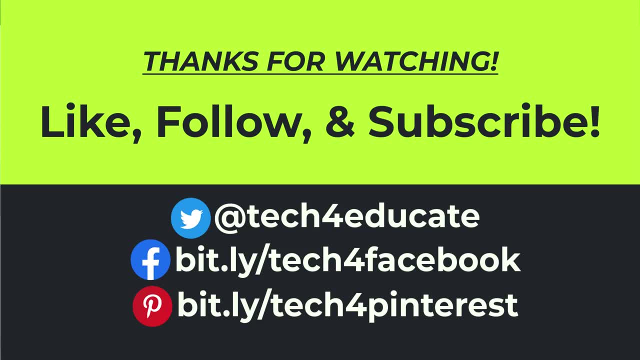 data that they're looking for, while ignoring the other data, at least temporarily. Thanks for watching. I hope you found this tutorial to be helpful. If you did, please like, follow and subscribe, And when you do, click the bell so you'll be notified when I post another video. 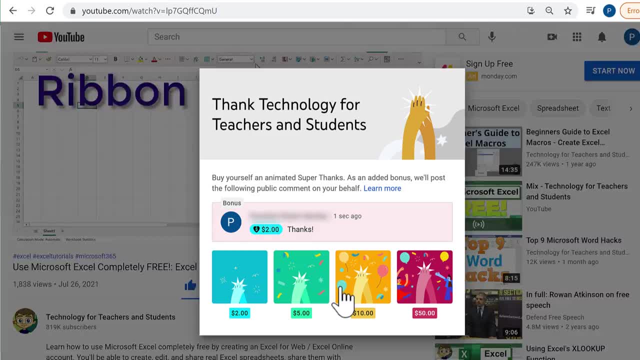 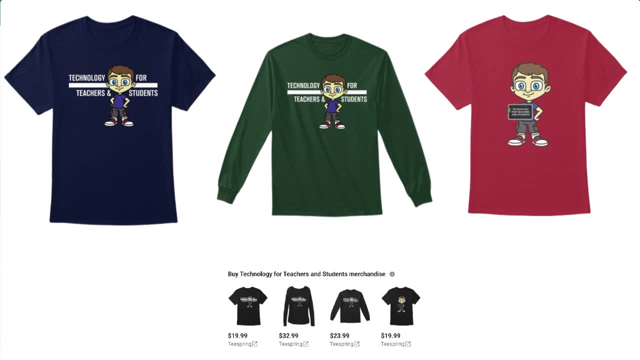 If you'd like to support my channel, consider clicking the thanks button below the video, or you could support me through my Patreon account or by buying channel merch, and you'll find information about those options in the description below the video. If you're new to Patreon, I want to give a quick shout out to my $5 Patreon supporters. 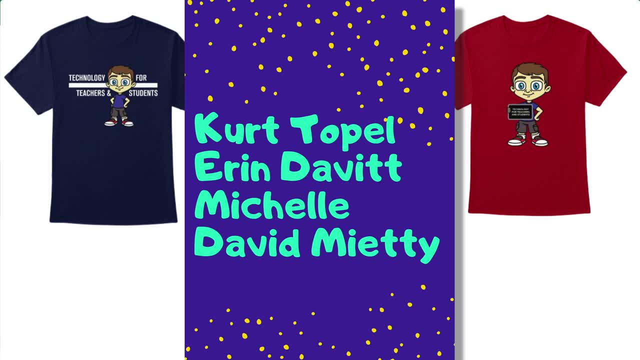 Thank you so much for all you do to support the channel. Without you, I wouldn't be able to post as many videos as I do, And I really appreciate, actually, all my Patreon supporters, not just at the $5 level. Thank you.